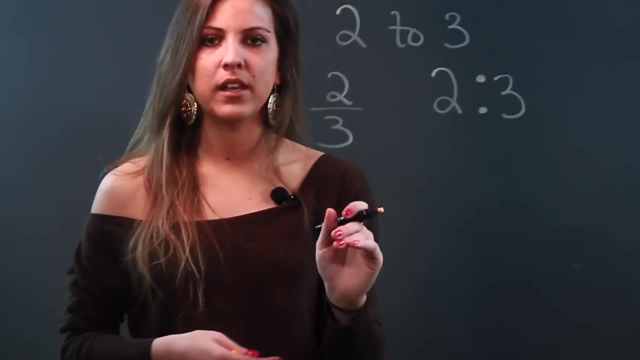 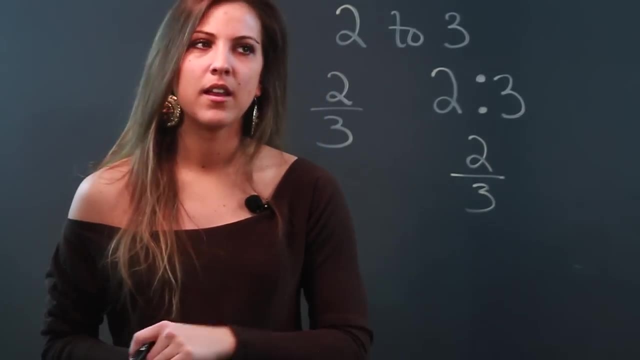 as 2 to 3.. So again, if you see it like this and you want to write it as a fraction, whatever the first number is, you simply put it in the numerator, and whatever the second number is, you just put it at the denominator. So we'll do one more ratio. Let's say I had 5. 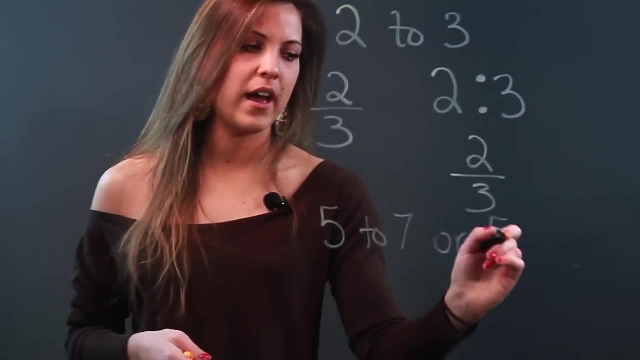 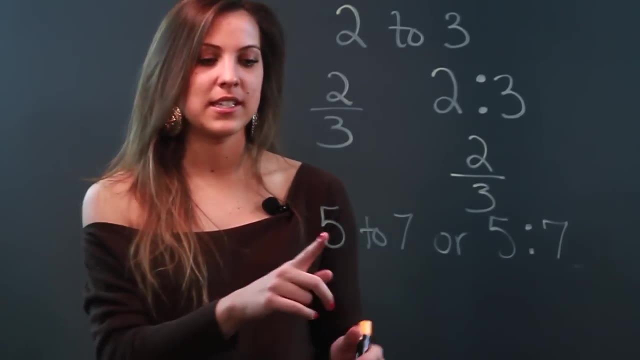 to 7,, or it can be written 5 to 7,, or the third way to write it is the way that you want to write it as a fraction. Again, I'm just taking the first number. whatever it is, it's going in the numerator and whatever. 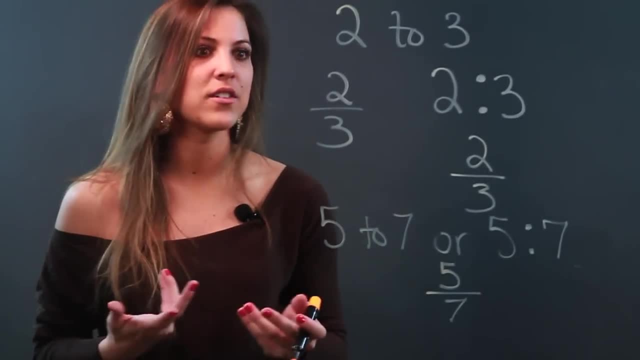 my second number is: it's going in the denominator And that's all there is to it. That's how you write a ratio as a fraction. 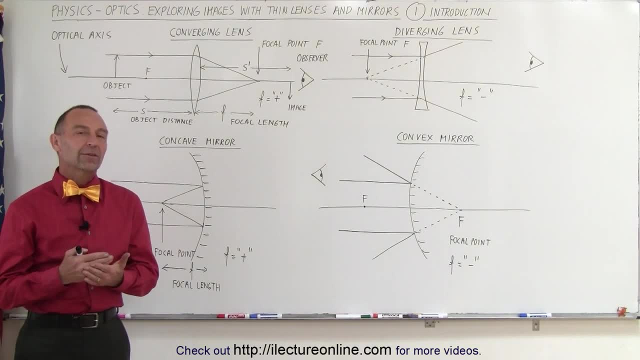 Welcome to Electron Online. I get a lot of questions about mirrors and lenses, Questions such as what happens when the object is placed at the focal point, what happens when you move it to the left, move it to the right things like that, And I thought it might be a good idea to put. 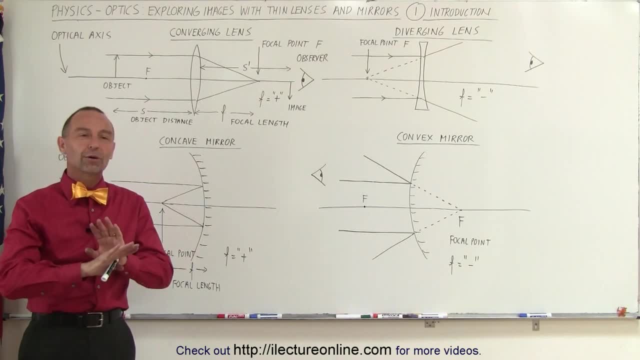 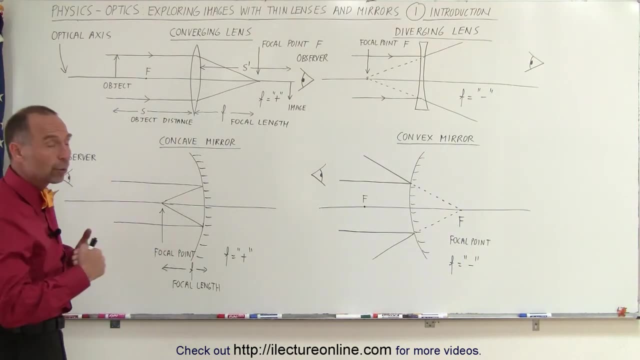 a set of videos together to explain some of these things in a more general aspect, more general perspective. So that's what we're going to do here, starting with this first video. So, first of all, what we're going to be talking about is two types of lenses: converging lenses and diverging. 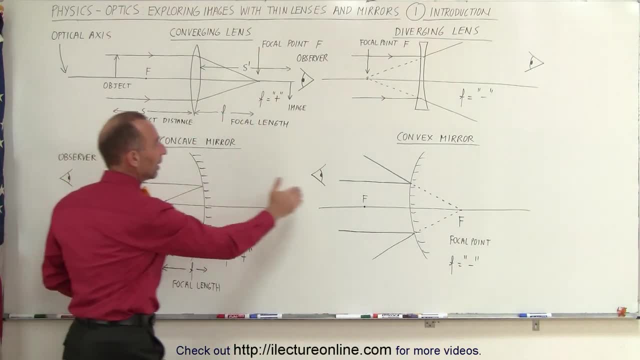 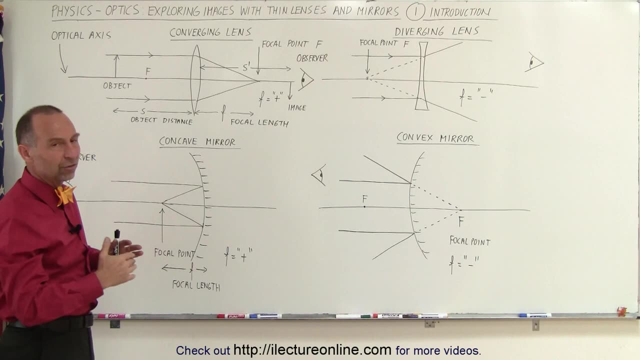 lenses and two types of mirrors: concave mirrors and convex mirrors. Now the lenses are what we call thin lenses. Later on we'll do some series on thick lenses and those are very different. So what are some of the major aspects, some of the key aspects that we have to know about lenses? 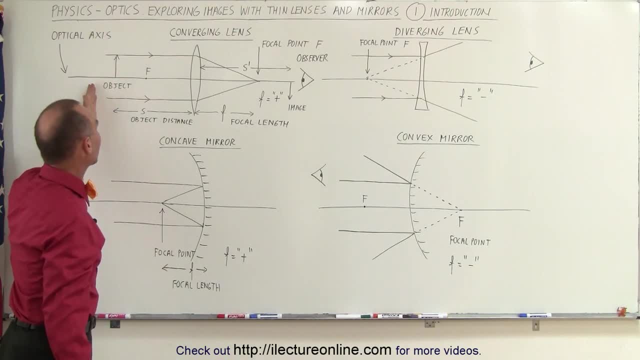 Well, first of all, typically we place the object to the left of the lens and the observer tends to be to the left of the lens. So we place the object to the left of the lens and the observer tends to be to the left of the lens. So we place the object to the left of the lens and the observer